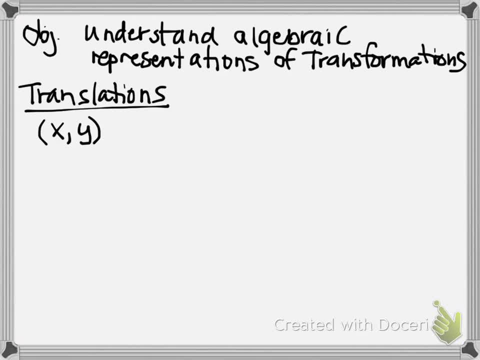 We're just going to use variables to represent rules And we have different combinations that can occur, So I'm not going to write four different, because there's actually four. There's actually four different combinations we could have. I'm not going to write them all out, I'm just going to write one generic one and then talk about it. 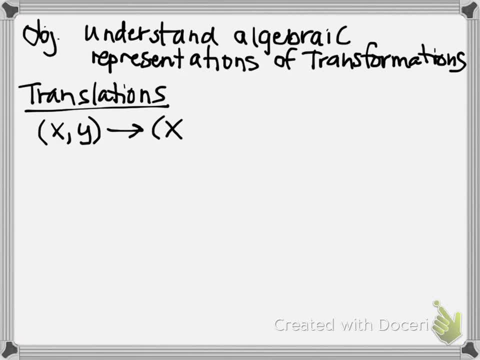 If we're going to move an object and we want it to move an x value, we're going to take that x value and we're going to say it's a and we're going to add it. Now we're going to talk about how a could be positive or negative. 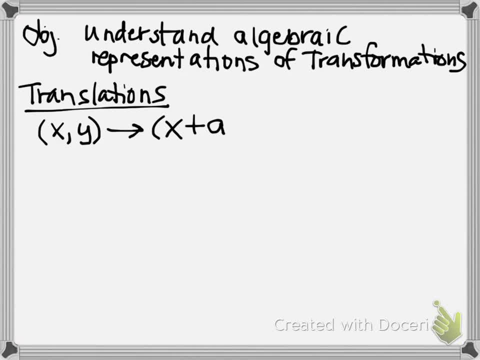 Okay, so that's going to explain what the actual physical move is going to have. And then we had talked about with the y value we're going to add some sort of b value. So let's kind of break down what could happen. 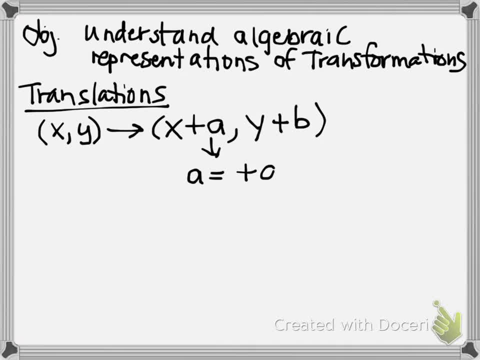 A. A could be a positive a if the directions tell you to move where Right, Okay. So this would give you move right a places, Okay. But if, If we get a negative a, what is that going to tell you to do? 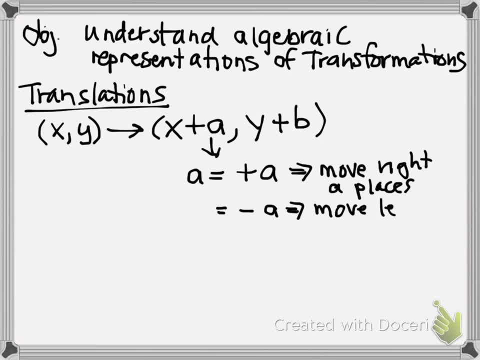 It's going to tell you to move the other direction, move left a places. Now, with some translations, that's all it was. It was just moving right or left. That's all they wanted you to do. Okay, Some translations wanted you to move only up or down. 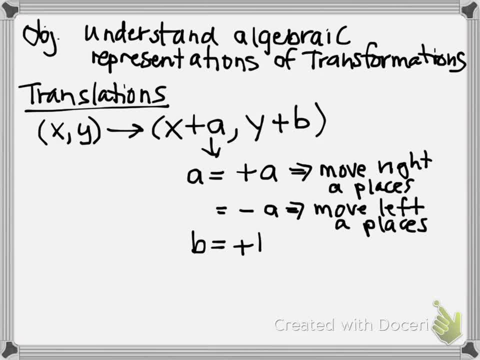 And that's the b value. So if it was a positive b value, what direction did you move Right? Okay, We can't go right in two different letters. We can only go one direction. So we're going to move up because it's positive. 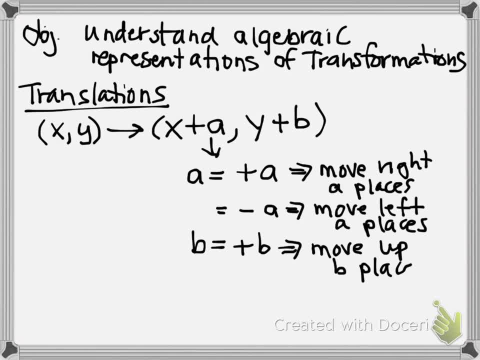 B places, And if it was a negative b you would move down that many places. So again, when we were doing our translations, we either didn't If we did just an x shift, like from quadrant one to quadrant two. 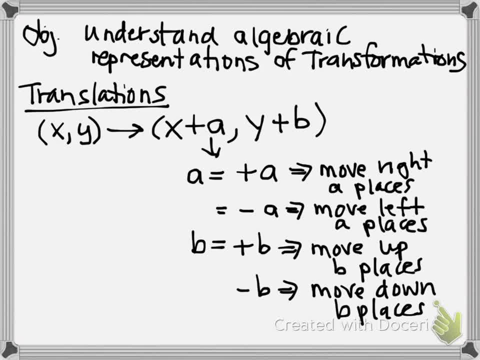 or we did a y shift, so let's say sorry, I did that wrong. If we did an x shift, we would do quadrant one to quadrant four. If we did a y shift, we would do quadrant one to quadrant two. 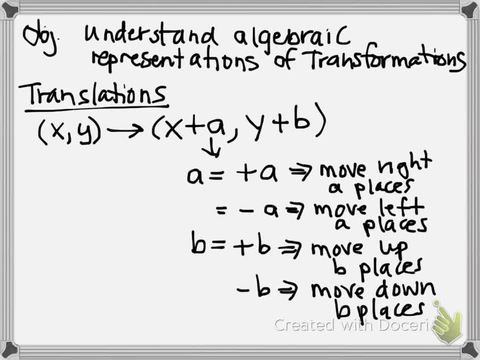 And then there were times where we did both an x shift and a y shift, so like quadrant one to quadrant three, So that would be a diagonal shift of some sort. Okay, So you could do it individually, You could do it in combination. 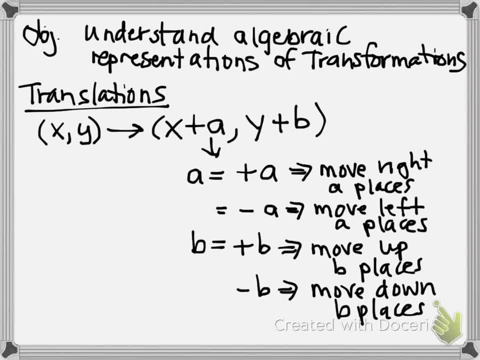 Okay, And so we had all those different scenarios And where- Let me add this back in here- You guys have got the packet you can get into the online book, So I attached to your packet lesson 9.4.. So there's an example of this. 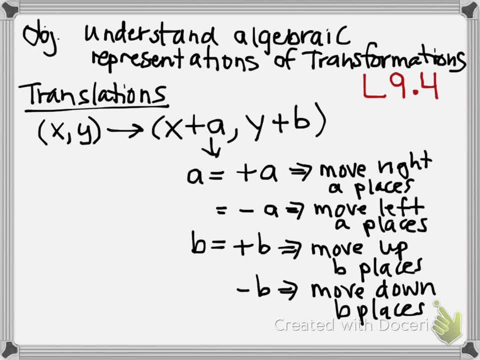 Okay, So you can look through the examples yourself And also with each of the examples. if you look here at the Your Turn and you're online, you can go to. I'm a personal math trainer and so that's really good, okay. 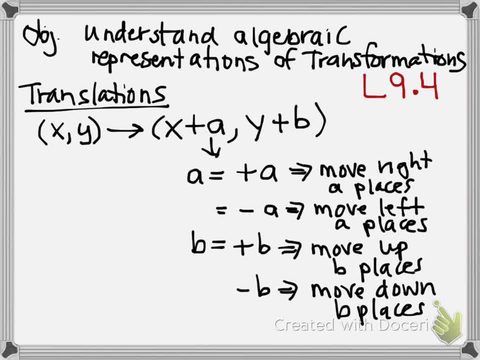 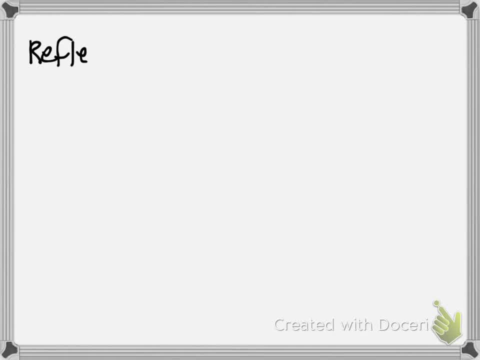 Then let's talk about rotations or not rotations. let's talk about reflections. So reflections, You had different sorts of movement, but it was always over an axis. Now you can reflect over any line you want. You could reflect over the line x equals one. 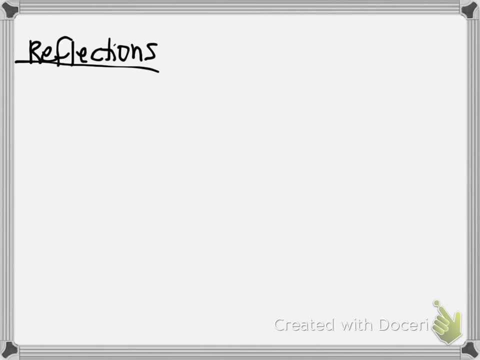 You could reflect over the line x equals one. You could reflect over the line y equals two. It doesn't matter, But we're only focusing in on reflecting about an axis. okay, Kaylin, wake up, sweetie, Okay. 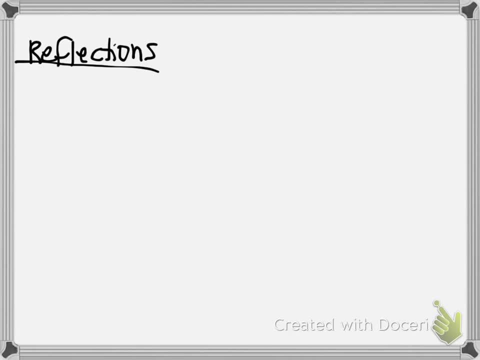 So we had two types of reflections, right. We could reflect over the y-axis or we could reflect over the x-axis. So let's deal with each one. So reflect over x-axis. So let's draw a quick picture without my fancy stuff. 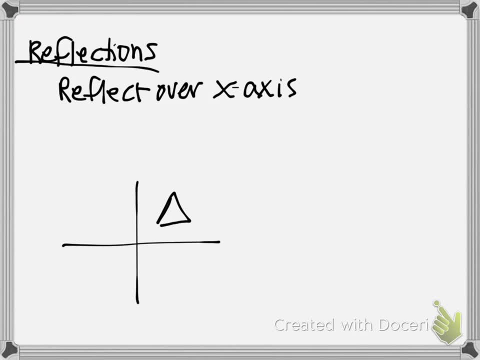 So if I'm reflecting over the x-axis, I'm doing this okay And what I would start with is my original ordered pair. But what would I do? What would change in that reflection? One, Two, Three, Four? 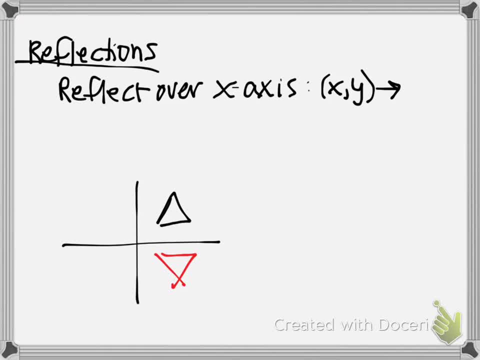 Five, Six, Seven, Eight, Nine, Twenty, Thirty, Fif, Twenty, Twenty, Twenty, Thirty, Twenty, Twenty, Fif, Thirty, Twenty, Twenty, Twenty. Look where your x's are and look where your y's are. 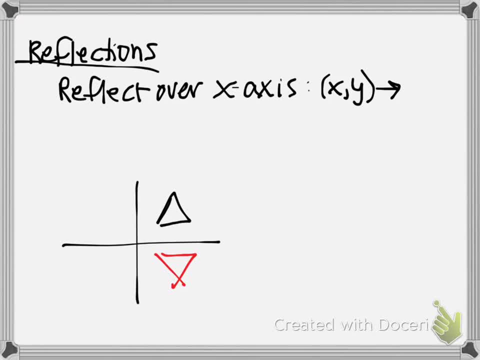 And what is the actual change with those ordered pairs, Ryan, you remember? Okay, so in this one, who becomes the negative, The x or the y? Okay, so when you reflect over the x-axis, you now have negative. oops, sorry, that wasn't the color I wanted, sorry. 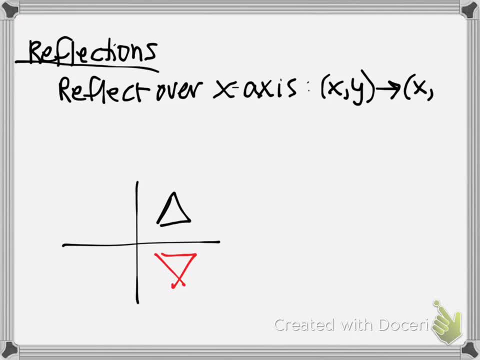 Oops, I'm supposed to be erasing. Now we can do that. You have a negative y, So you're going to multiply the y by negative 1.. The x value will stay exactly the same. It's the y value that's going to change. 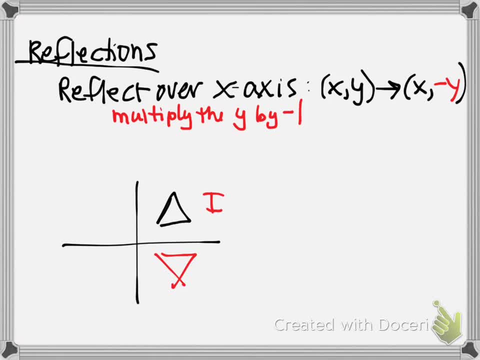 Because you can see in that picture, you go from quadrant 1, to quadrant 4, and in quadrant 4, your y's are negative. So you have a positive x and you have a negative y. Quadrant 1, you had positive, positive. 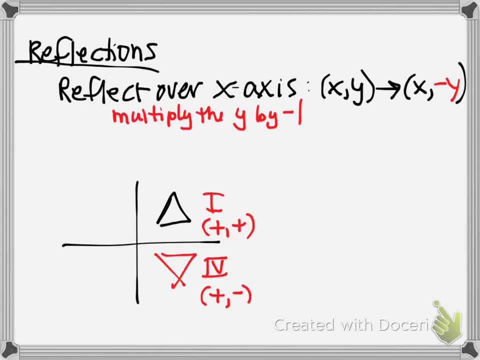 So it doesn't matter where your shape is. Anytime you're reflecting over the x-axis, your x is fine. It's your y that changes to the opposite sign. So then the other option would be to reflect over the y-axis. 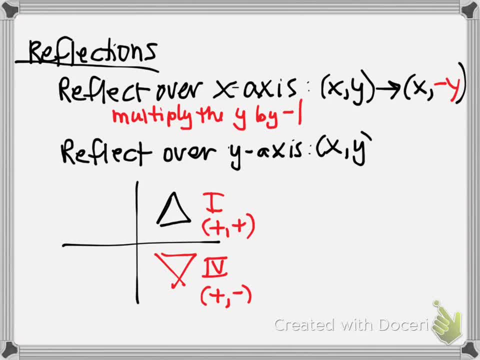 So again, here's your original point. So let's say that we're going to reflect over the y-axis on this one. okay, And now what's going to change on this shape? Okay, what's going to change on this shape? 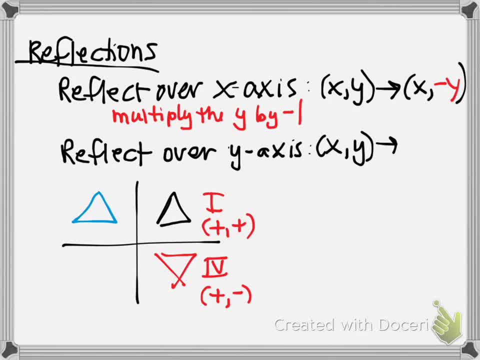 I only have one answer, man, today. right, The x will be negative and the y will be positive. Yeah, what happens is now I'm still at the same level as the other shapes, so the y hasn't changed, but what has changed is my x value. 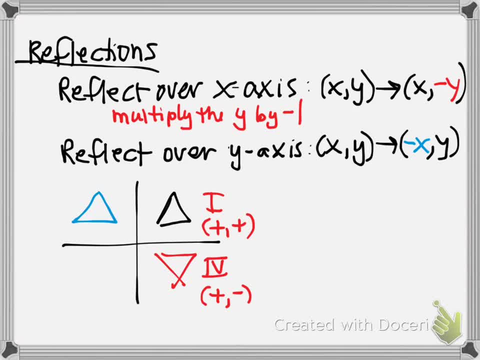 So we're going to. anytime we're told to reflect over the y-axis, we're going to multiply. oh man, Sorry. We're going to multiply the x by negative one. okay, So I can mathematically already know what my ordered pairs will be. 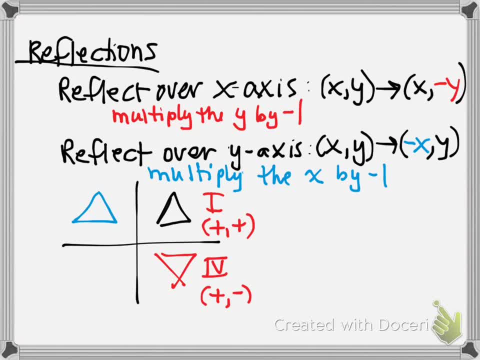 and that will help me get where I need to go. Boy, we've got two sleepy girls right there. Wake up there, Samantha. Oh my goodness, the two of you together, Woo-hoo. Okay, And again in your packet you can look at the example of that. 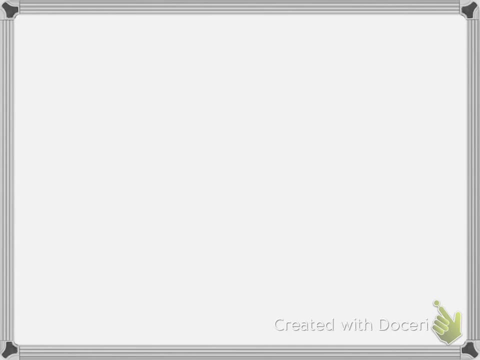 Here comes the fun one: Rotations. Oh, I'm sorry. So now let's talk about rotations, And with rotations, what it boils down to is: what direction are you heading? Okay, If you're going clockwise, we have one thing that changes: 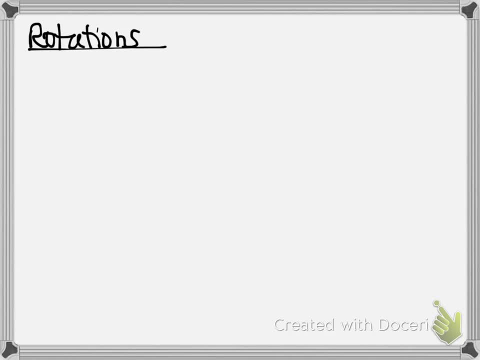 If we're going counterclockwise, it's another thing that changes. So it's the direction that you're heading that's really going to determine how we're going to go. So if we're going counterclockwise, it's going to mathematically change. 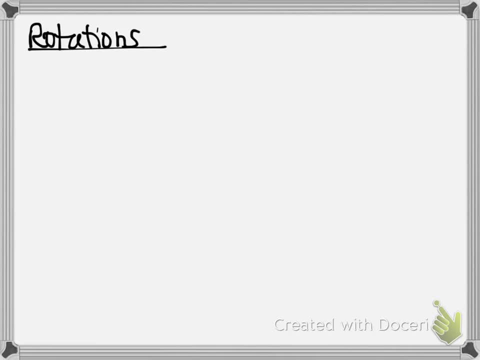 So let's deal with clockwise first And we'll just deal with 90 degrees clockwise. So clockwise is to the right. What happens is that you're going to take your ordered pair and two changes take place. Change number one: we're going to the left. 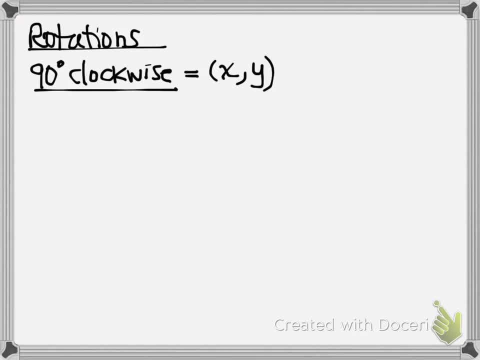 Change number two: we're going to the right. Change number three: we're going to the left. Change number four: we're going to the right. So we're going to take our x value and you're going to multiply by one. 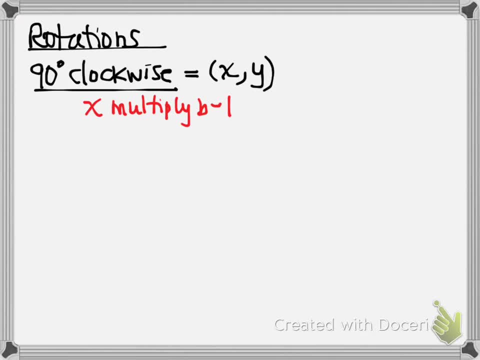 Or negative one, sorry. Second thing that's going to change is you're going to switch x and y. So what we end up with is we're going to take the x value and multiply it by negative one. Y comes in front. So the original y-coordinate- listen up, Connor- becomes the x-coordinate in the rotation. 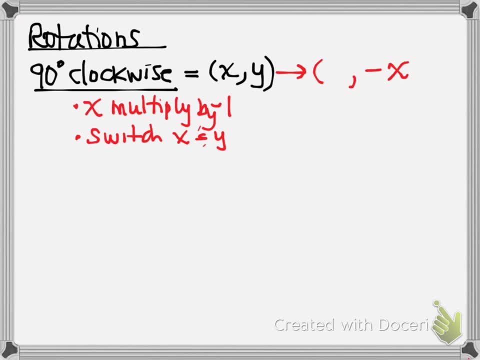 Okay, And the original x-coordinate gets a, negative, times it and then it becomes the y-coordinate. That's the weird piece. All right, Let's go the other direction: 90 degrees counterclockwise. So we're going to do the y-coordinate. 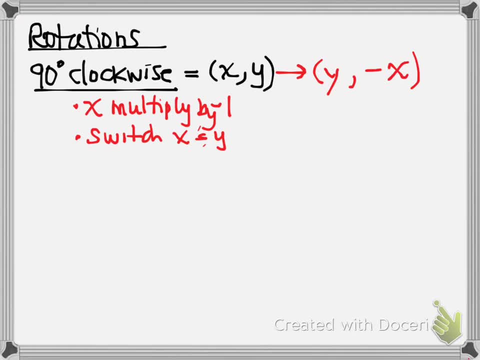 And the y-coordinate is that Theниц x And the original y-coordinate comes in front of it And then the y-coordinate gets a negative divisor. All right, So this is the y-coordinate And then you have the y-coordinate that's going to get a negative divisor. 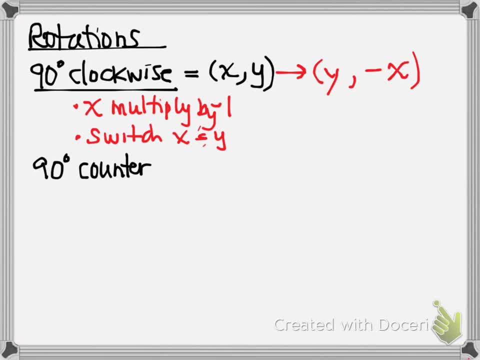 So that's the y-coordinate. All right, Now let me show you Counterclockwise. Now again, all of these. we're going to be using the origin as our rotation point. So again, we're going to start with this ordered pair. 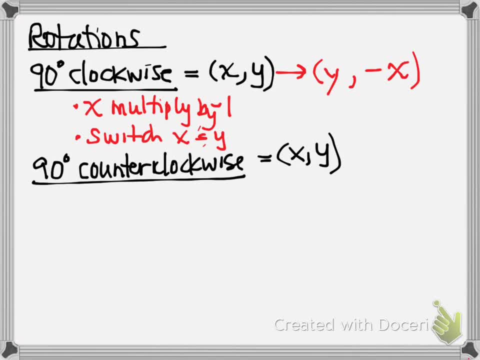 What do you think? we're going to multiply by negative 1?? We're going to multiply the y by negative 1.. And we're still going to do the switching: Switch x and y. So this, when I rotate it counterclockwise to the left: 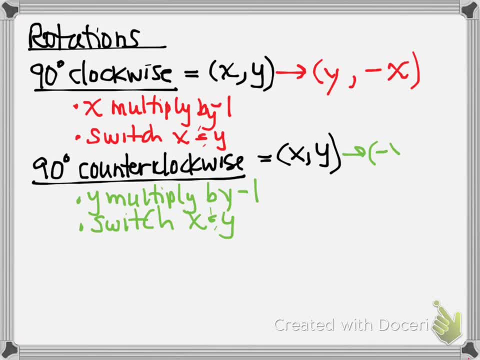 we're going to multiply the y by negative 1, and it now becomes the x value, and the old x value becomes the new y value. Okay, Now the other one is the 180 degrees rotation. So what do you think happens with the signs then? 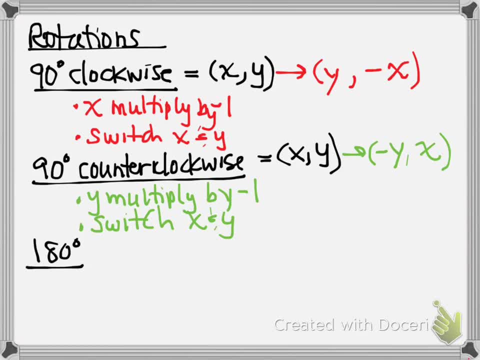 Think back to our homework. When we go from here to here, what's going to happen to these values versus these values? What's happening to your x's and y's versus these x's and y's? Okay, So both of them become negative. 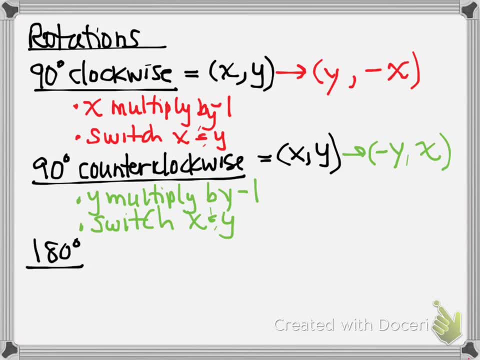 We multiply by negative, We're going to apply both of those rules and then they stay in the same position. So we're going to multiply both x and y by negative 1. No switching Because, if you think about it, if we've already made a comment that this is a double reflection, 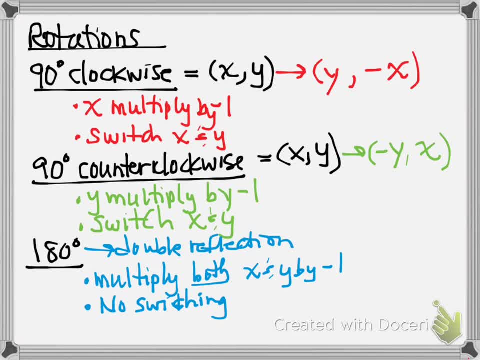 never in a reflection did x and y coordinates change spots right. So this one says: if you start with the order pair x- y, what you're now going to have is negative x, negative y, Okay, Okay, So the next.